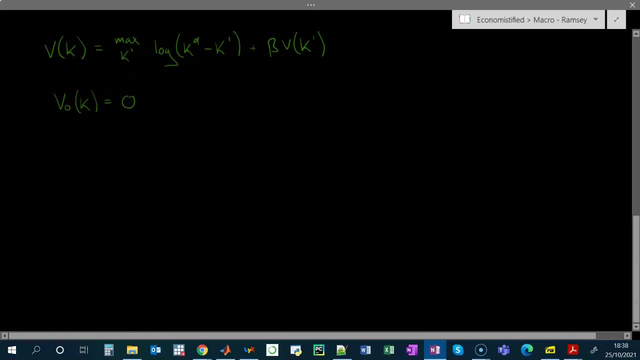 is that the value function is just equal to zero. Clearly, this is not a correct guess. We know what the correct guess looks like. We just found it in the previous video, But I'm going to plug this in nonetheless. OK, So plugging in my initial guess: zero on the right-hand side. I'm just going to get. 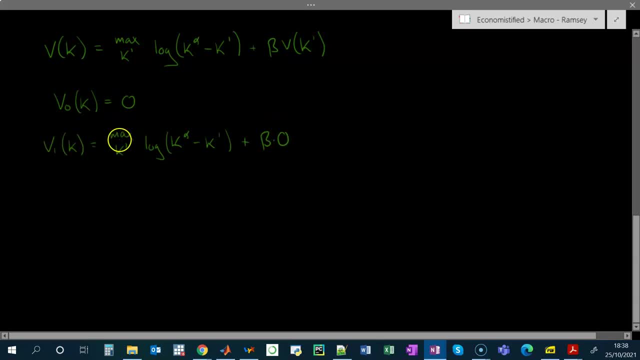 beta times zero. And so the Bellman equation says that my current utility is given by the log of consumption. But there is the continuation value, So all the utility I get after the current period is zero by assumption. Now let's find my optimal choice of capital given this guess. Well, clearly, k prime only. 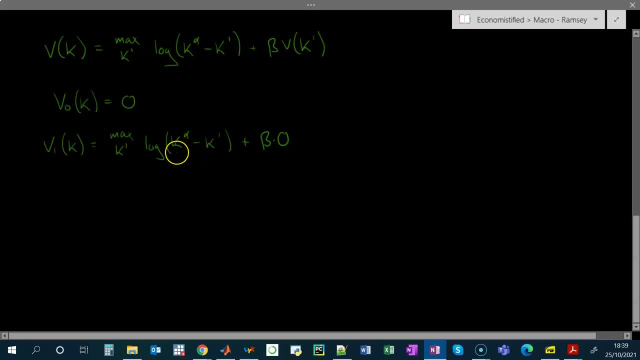 appears once here and it appears negatively. If I reduce my consumption today and save more, I'm going to reduce the utility I get from consumption today. Now, ordinarily I would be able to use those savings later on and consume them later on and get some utility. 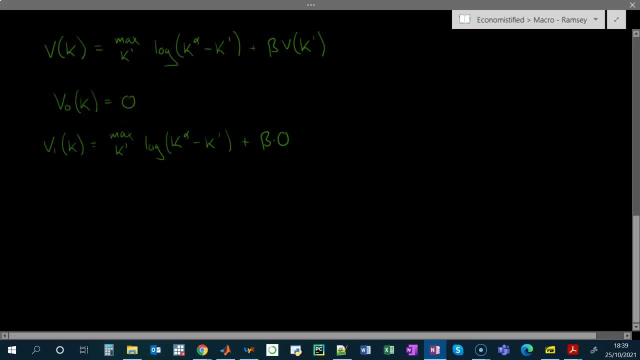 then. But I'm assuming With my guess that the utility from that is zero. So I'm assuming there's zero here. So obviously my optimal choice of capital here- and I'll call this k zero prime, because it's my optimal choice of capital given my zeroth guess- my optimal choice of capital. 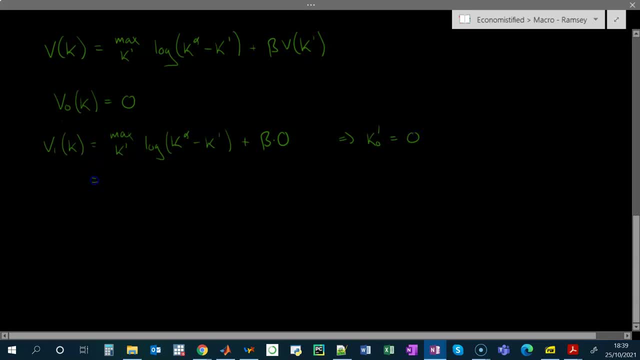 is going to be zero. OK, Now let's plug in my initial guess and my optimal choice, given that guess, back into the Bellman operator, into the Bellman equation And what I'm going to get out, I'm going to use as my new guess the 1k. So, plugging in this k zero prime, I can get rid of the max. 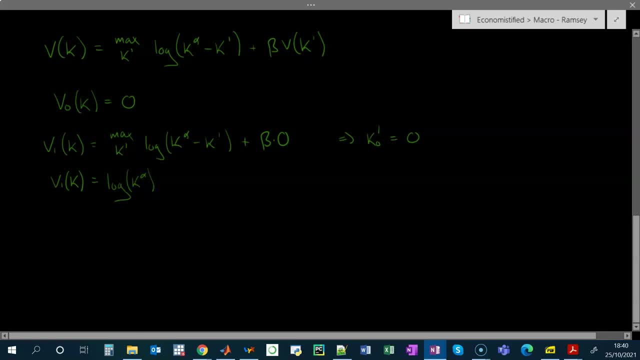 operator here- And I just get the flow utility- is the log of k to the alpha, because k prime is zero And then this beta times zero is obviously just zero. So this is my optimal choice. So this is my second guess for the value function And it's equal to alpha log k, which is still 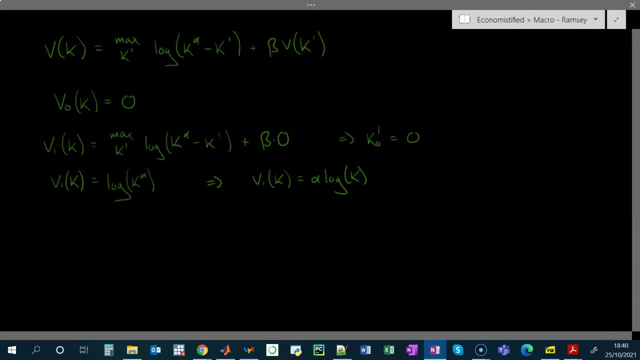 incorrect. We know what the true value function looks like. It has a constant term and the coefficient on log k here is not quite right, But it does have the same functional form. In other words it's proportional to the logarithm of k. 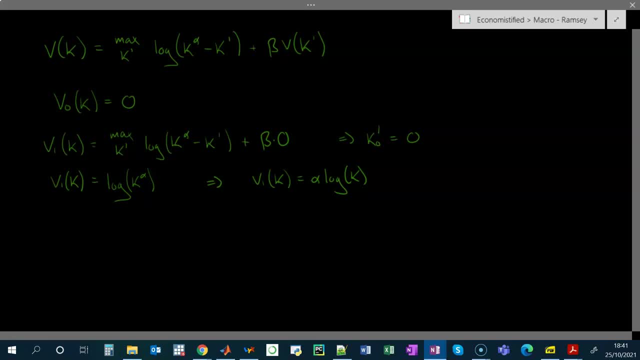 So even after just plugging in the k zero prime, I can get rid of the max operator. So even after just one iteration, value function iteration has proved fruitful in that it's now allowed us to find the correct functional form for the value function We don't know. 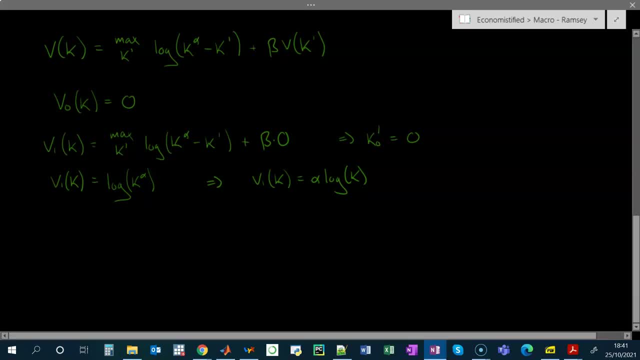 that yet We only know that because we already found it in the previous video. But as we keep iterating, I plug this v1k in as my new guess. we're going to see that eventually we get the true value, So let's plug v1k in. 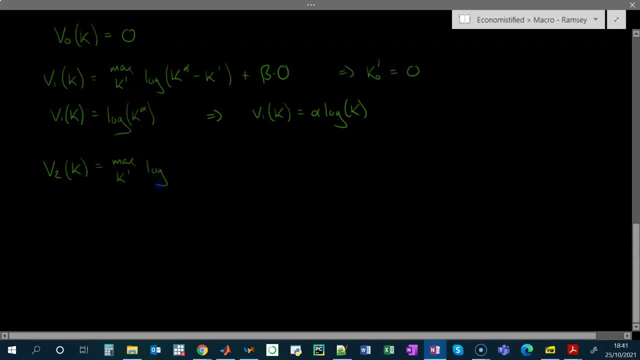 v1k into the Bellman equation again. And now, instead of having v to zero, I'm going to use my new guess for v v1, a alpha log k. Let's find the first order condition again. So taking the derivative with respect to k prime gives me this: 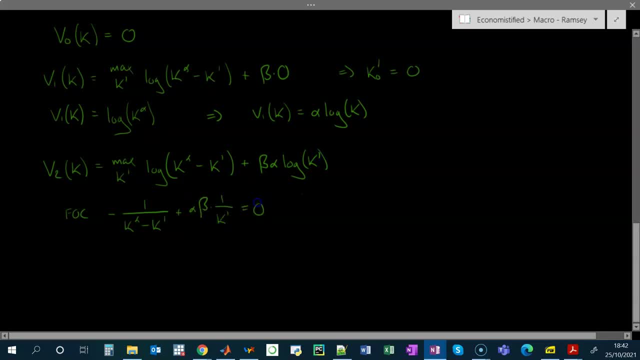 k should be prime, of course, And my optimal choice of capital, given my second guess for v, is going to look like this. So this is still not the correct policy function, as we know because we know from the previous video, The true policy function is going to be equal to alpha beta times output. 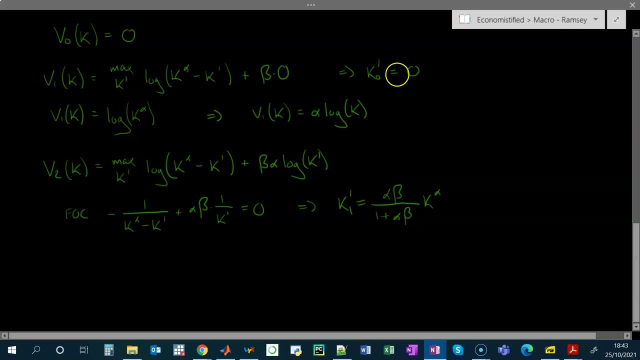 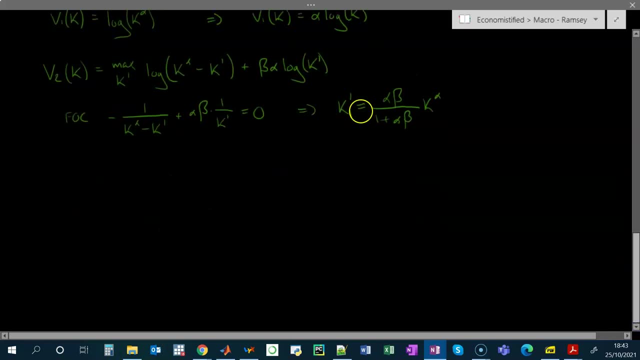 But it's certainly closer than the policy function that we found from the first guess. OK, Let's plug this k1 prime back into the Bellman equation. And what is the current value? 0.. OK, Sorry, Yeah, pretty good. 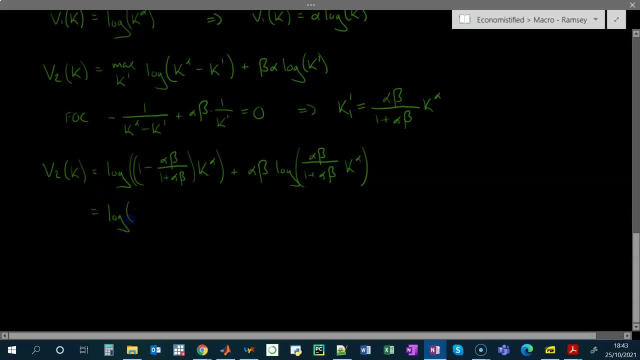 There we go. Looks like that. Can't get it to 0 again, But it's going to look like this: It should be equal to alpha beta times k prime over k prime, So let's plug that in, OK. And now, collecting the terms proportional to the log of k, we have something that looks: 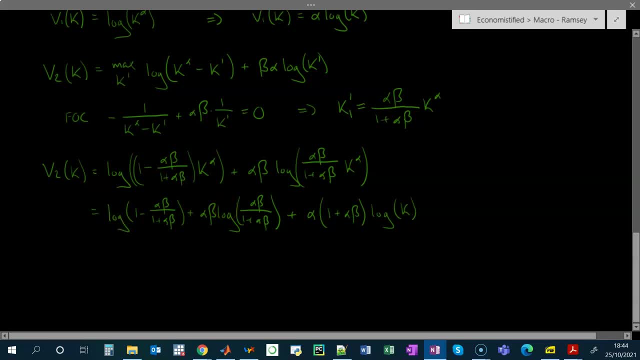 like this. Now I'm not going to bother with the constant again, just because that's a little tedious, But the term that is proportional to log k we now have looks something like this: constant plus alpha beta log k. Now, if I plug this into this v2, in as a new guess, 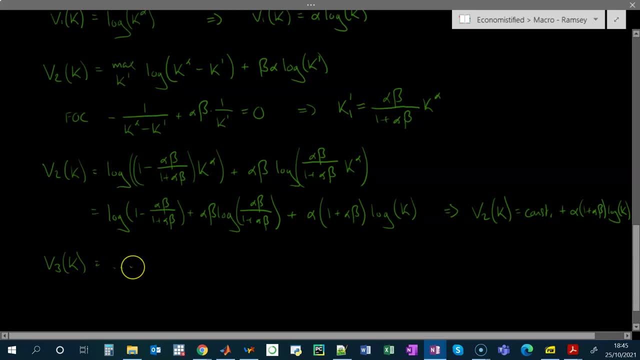 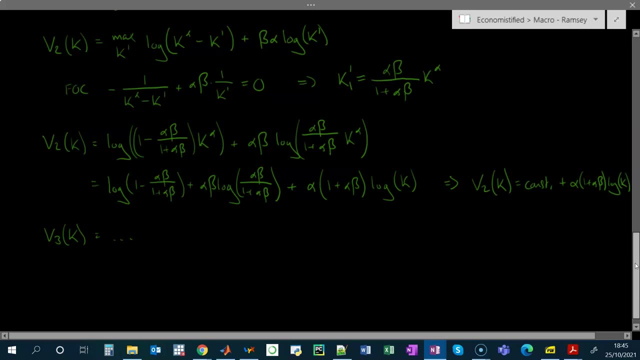 And find v3, I'm going to get something else. And if I keep doing this I'm going to get v4 and v5. And if I keep working out the policy function, I'll get k prime 3 and k prime 4.. 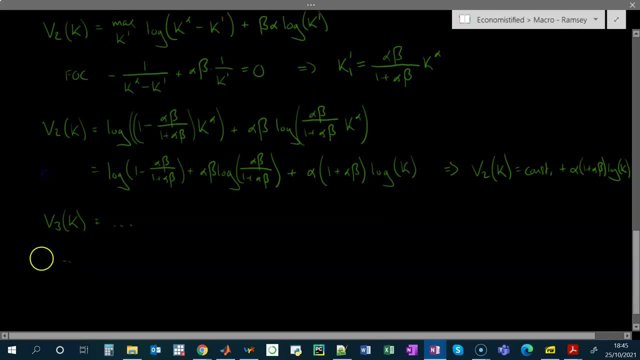 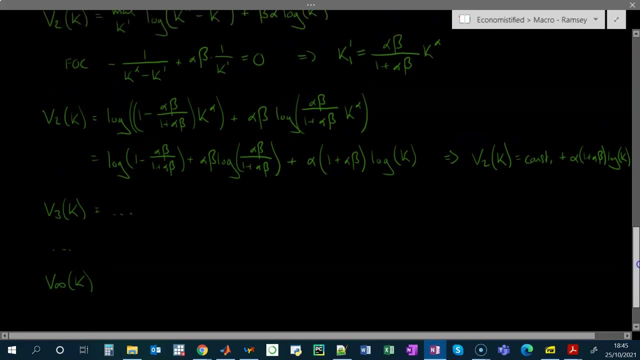 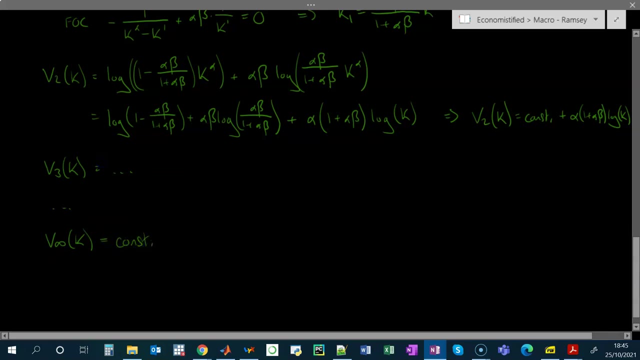 And if I do this ad infinitum, I'll get something like this, And you can kind of see the pattern here. hopefully, The infinite k, if you like, is going to. there's going to be something like this. It's going to be a constant term. 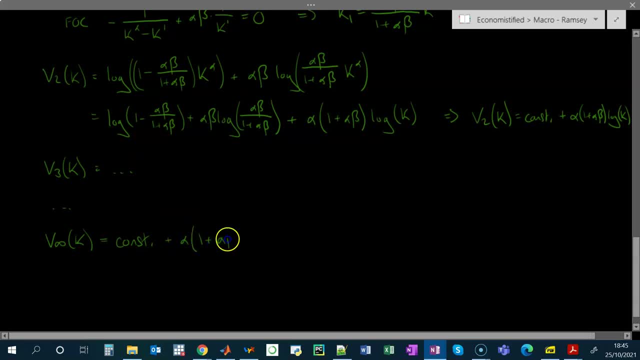 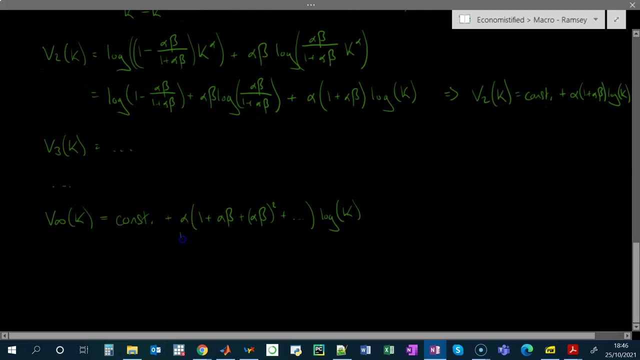 And then we're going to get plus alpha times 1, plus alpha beta, plus alpha beta squared, plus alpha beta cubed, and so on. log k, And if you remember your geometric series, you'll know that that is equal to alpha over. 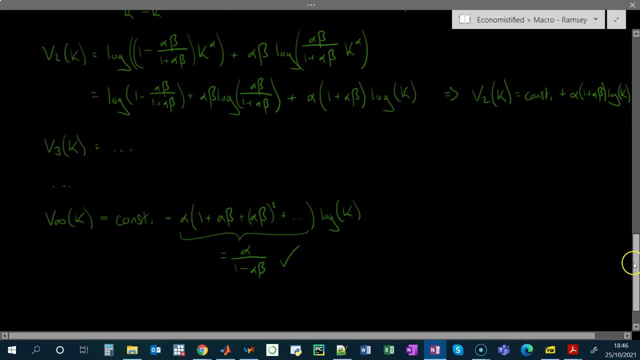 1 minus alpha beta, Which is the correct answer. Thank you, So that's the correct coefficient of proportionality on log k for the true value function. So I haven't worked out the constant, but you can take my word for it or you can work.